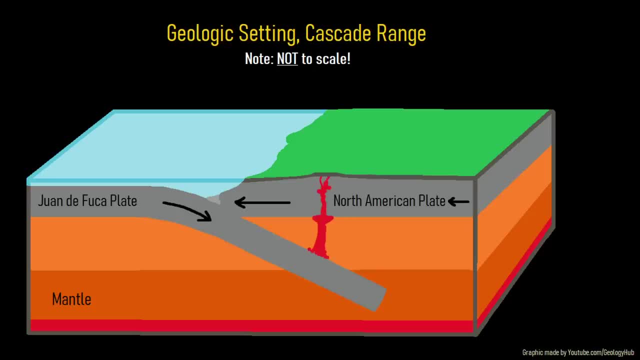 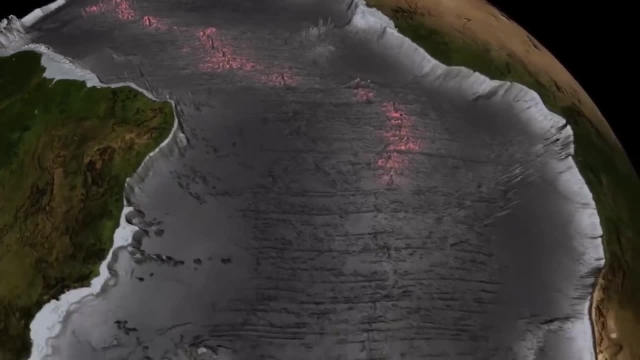 is created before eventually getting destroyed many millions of years later in a subduction zone. Earth has an estimated 65,000 kilometers in length of mid-ocean ridges, which create new crust which every year, on average, emplace 20 cubic kilometers of lava. that creates 2.7. 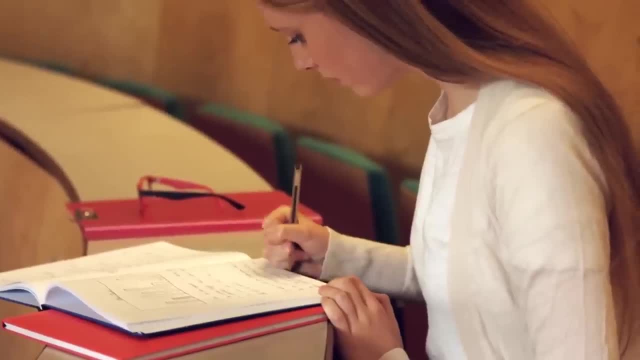 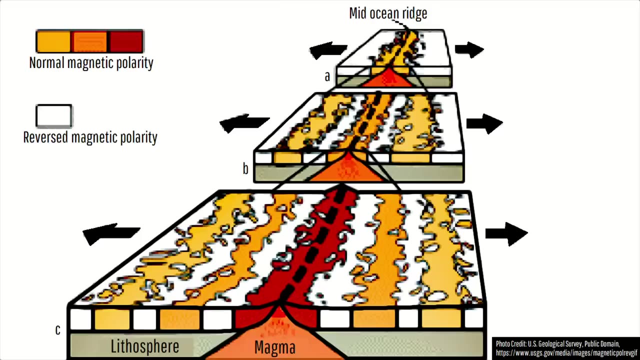 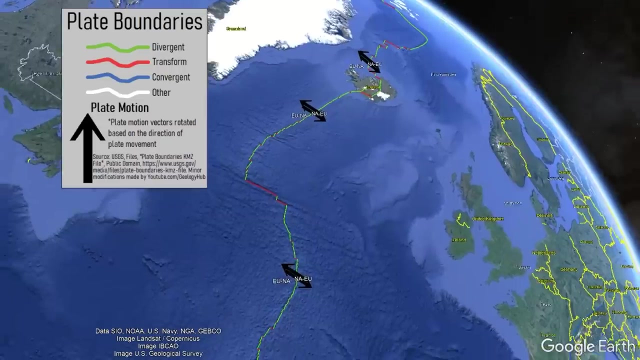 square kilometers worth of new crust. If you ever took a geology course in school, you might be wondering how exactly a mid-ocean ridge can only produce intermittent eruptions, as many textbooks display a mid-ocean ridge as continuously spreading apart. After all, the rate at which mid-ocean ridges spread apart each year is often cited as between. 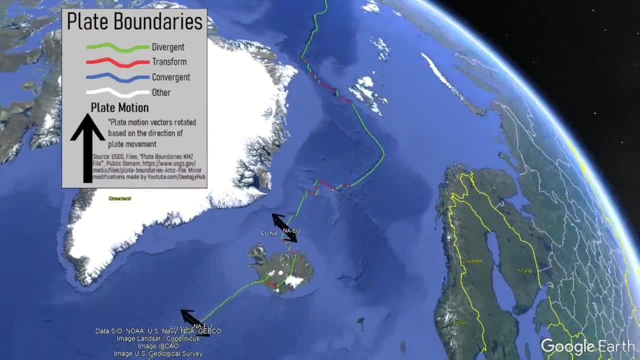 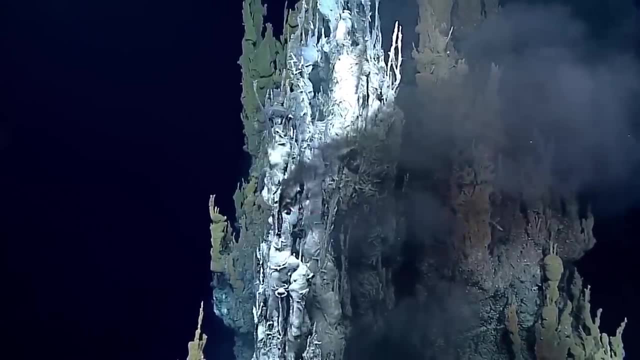 120 centimeters, depending on the exact tectonic plate boundary. While this figure is correct, it merely states a long term average. In reality, segments of mid-ocean ridges largely move in, geologically frequent, but space bursts of activity as stream is released. 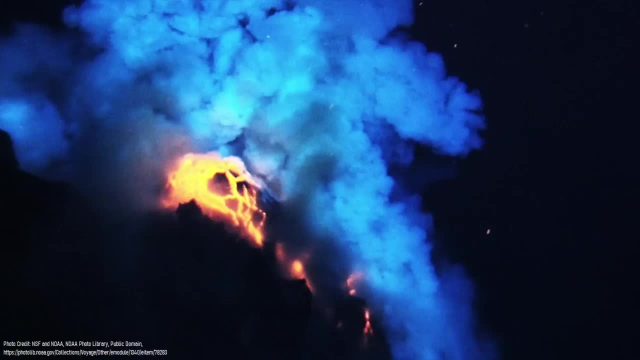 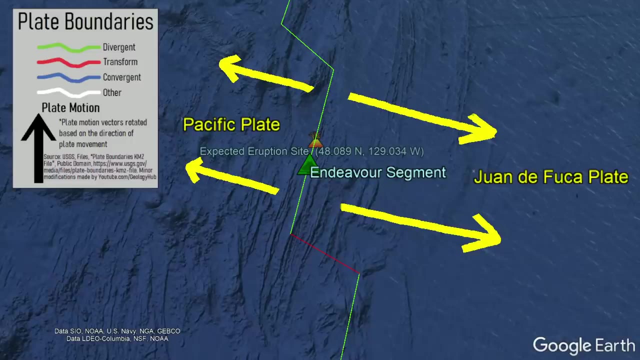 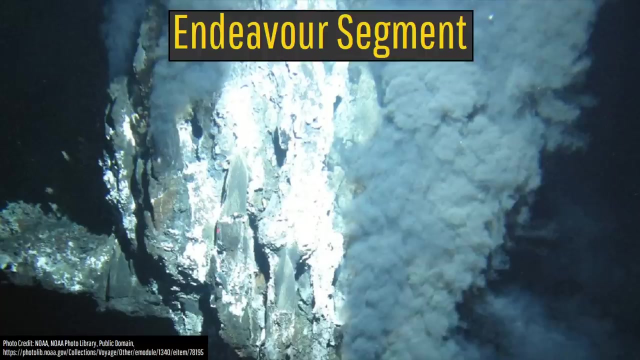 Meaning that sizeable underwater volcanic eruptions occur at a select few locations on these ridges every year instead of along their entire length, always erupting. In the case of the Endeavour segment, this mid-ocean ridge, which represents the diverging of the Pacific plate and the Juan de Fuca plate, last produced an eruption between 1999. 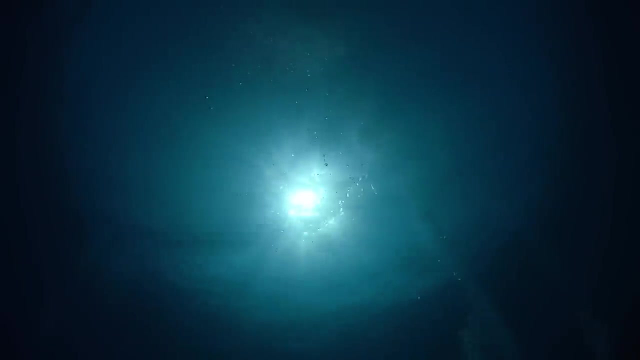 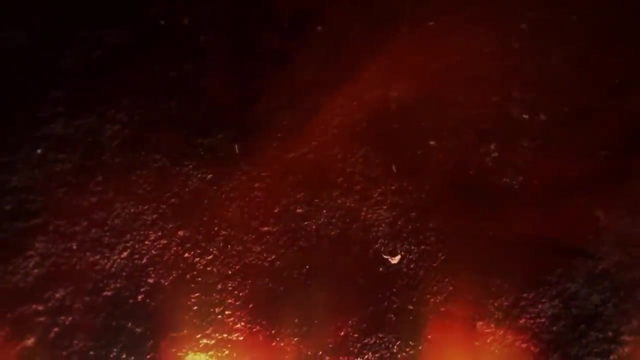 and 2005.. The earthquake swarm that was recorded on March 6th followed a slow but steady increase in activity from the same region, which began in 2019.. These earthquakes mark the release in stress and slow spreading of the crust, which will soon give magma a path to the ocean floor. 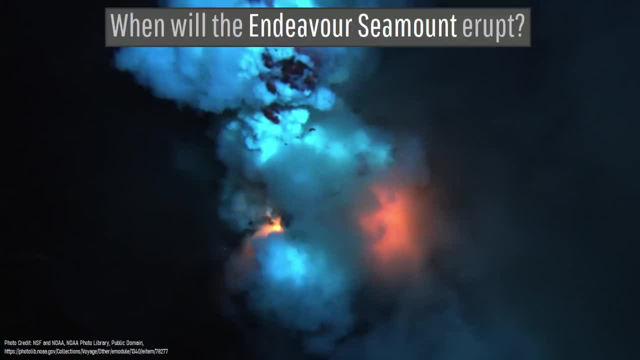 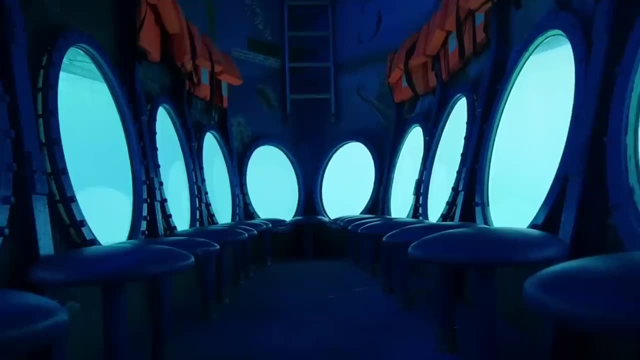 However, when exactly this seemingly inevitable eruption- which still might not occur, by the way- takes place, could range anywhere from a few days to several years from now. Yet if and when it does occur, scientists will likely visit the erupting region via 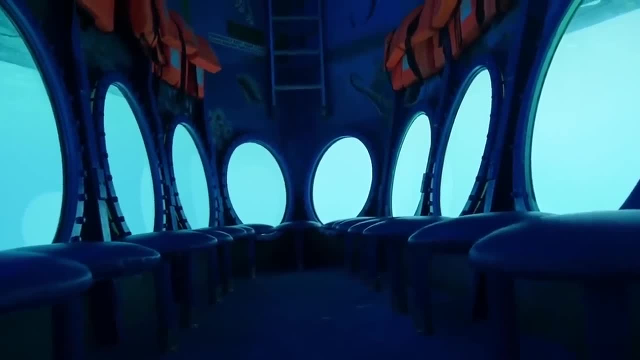 submarine to record a process which is not often directly witnessed. Mid-ocean ridge eruptions account for 75% of the total eruption area in the world, and the most recent eruptions were in the United States. In fact, the most recent eruptions were in the United States. 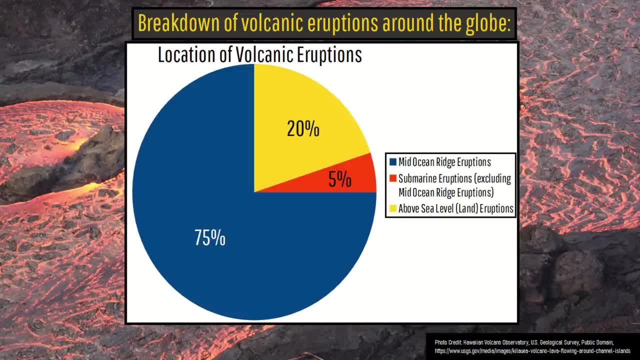 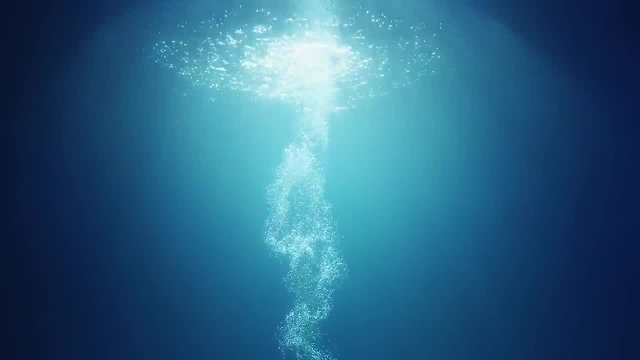 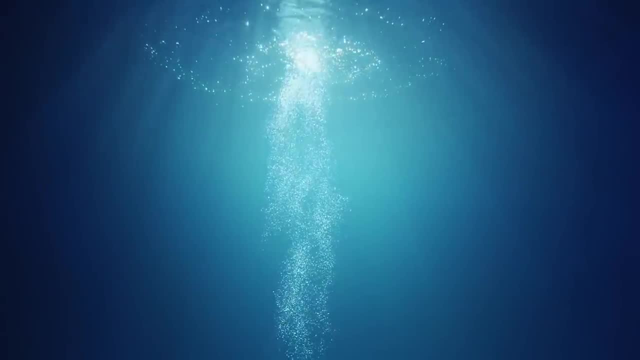 The 80% of submarine volcanic eruptions which occur each year and, due to their remoteness, are largely understudied. Thankfully, in my opinion, there are no dangers such an eruption will pose to anyone in the United States, Canada or beyond, due to it being completely effusive, confined deep underwater.